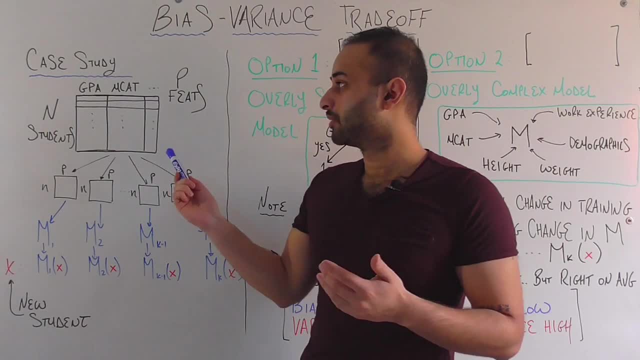 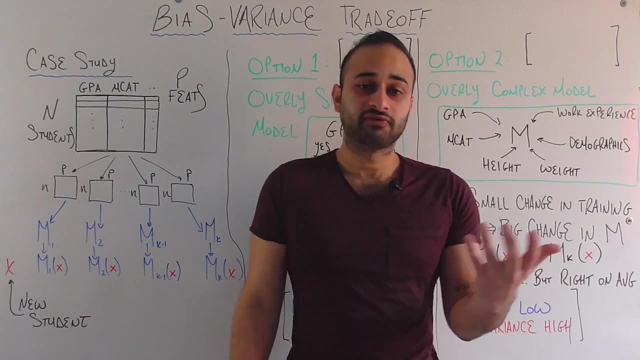 looking at any formulas. today, As always, we'll be going through a real world example and through this case study, I hope to more intuitively convey the idea of the bias-variance trade-off to you. and this is a very important concept because it does come up in practice. You have to think about. 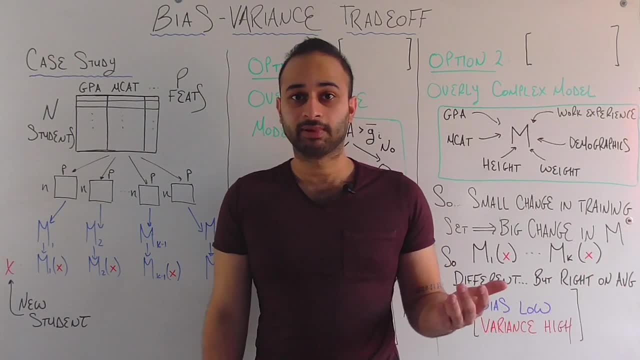 that when building your models, but also just speaking from a job, From a job perspective. it's something they love to ask during data science interviews. So let's get started. The real world example today is that you are doing a study on medical school admissions, So assume that this data set contains all of the students who applied. 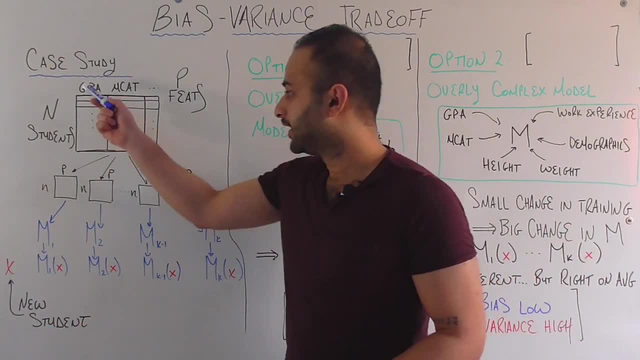 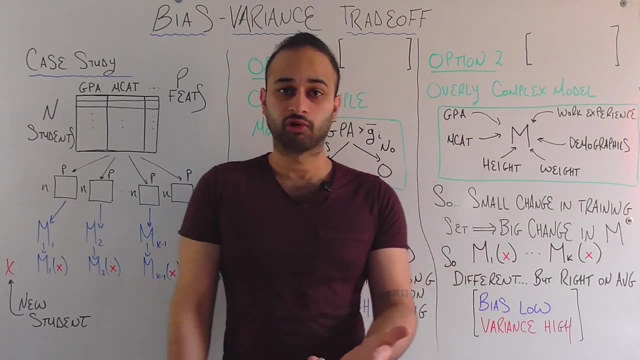 to medical school last year in the United States, for example. So we have n students, where n is obviously a very big number, and we have p features. So features are going to help us predict whether or not someone got into, let's say, their top choice: medical. 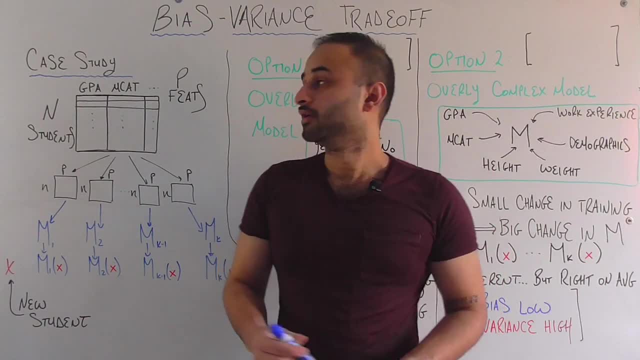 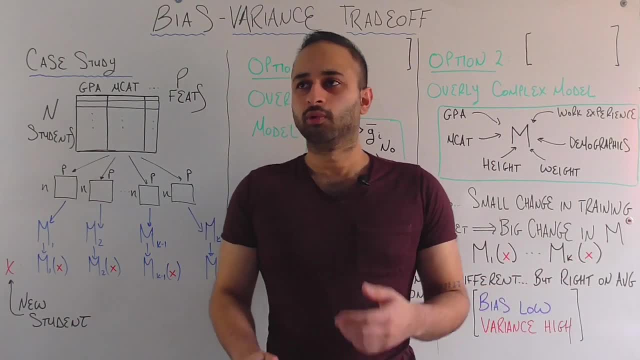 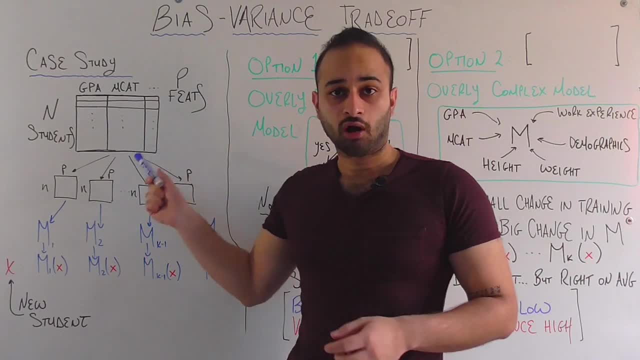 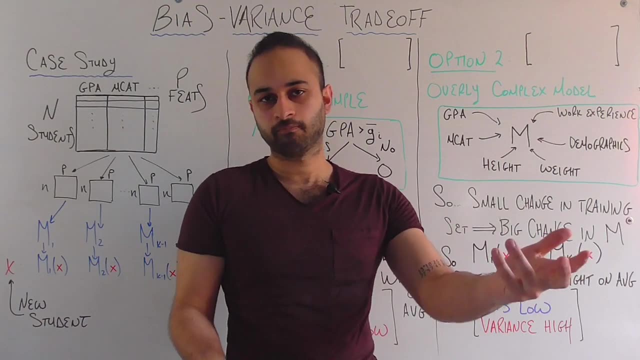 We have lots of things. Now, of course, you don't have access to all of this data. So you ask the medical board, or whoever supervises these admissions, to give you a small subset of the data, and they agree. So they agree to give you a small random subset of the data. 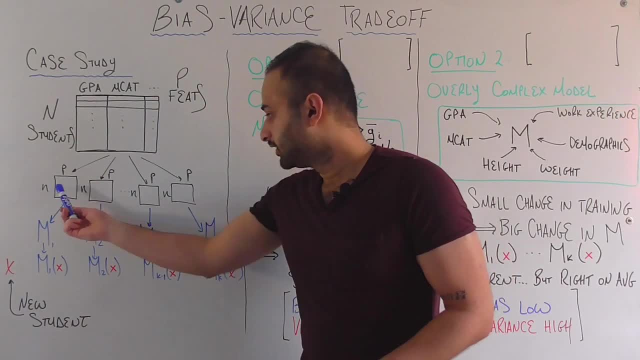 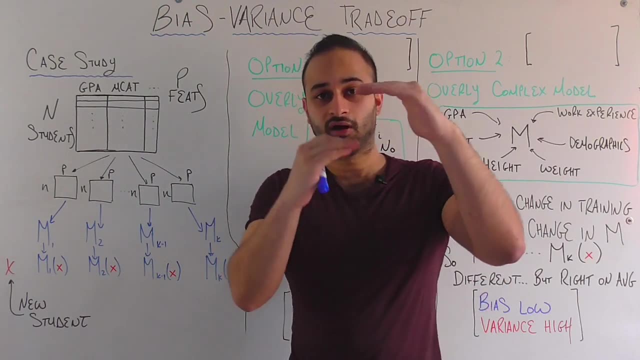 Now you don't know what that random subset is going to be. That's up to them. So you might get any of these k subsets here. So just to be clear, these are known as the rare. each of these is n by p little, n being the number of students they give you in. 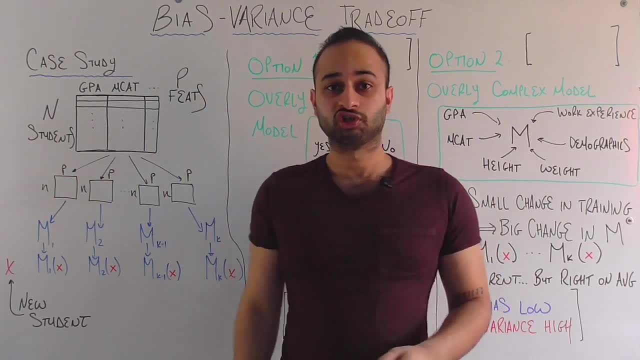 the subset, and this is random, and p is this number of features that we have. Okay, so you don't know which of these you're getting. it could be any of these, but you know you've got one of them and you know it's completely random. So now, 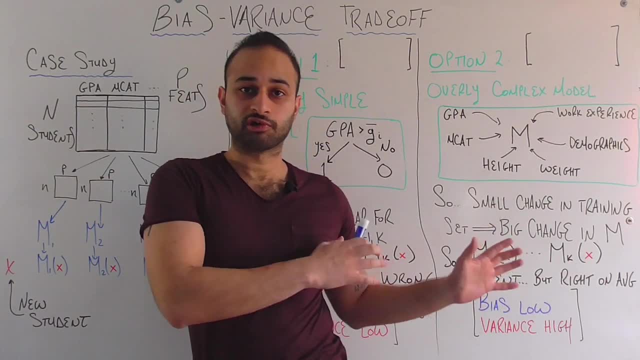 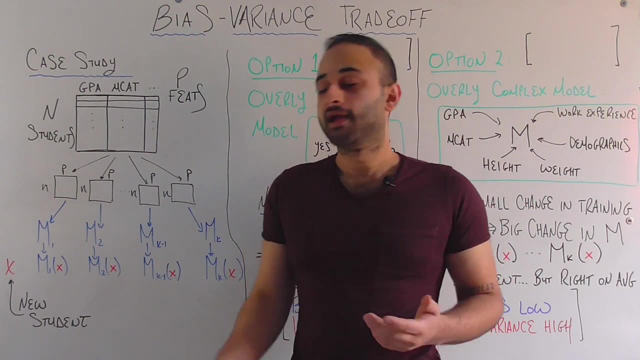 based on whichever one you get. you're going to build some model and we'll make those models more specific in a moment, but for now let's just say it's generally. you're gonna build some model: M1, if they give you this training data set 1,, M2, if they give you training data set 2, and so on, If they give you. 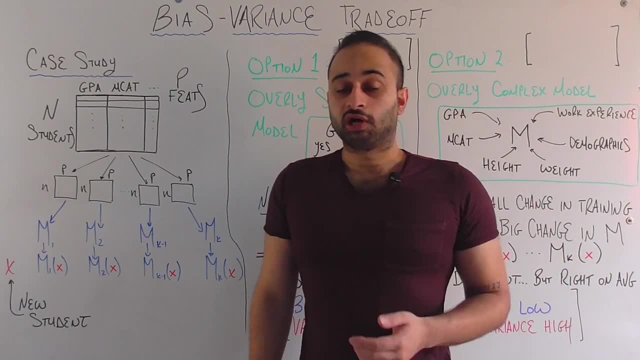 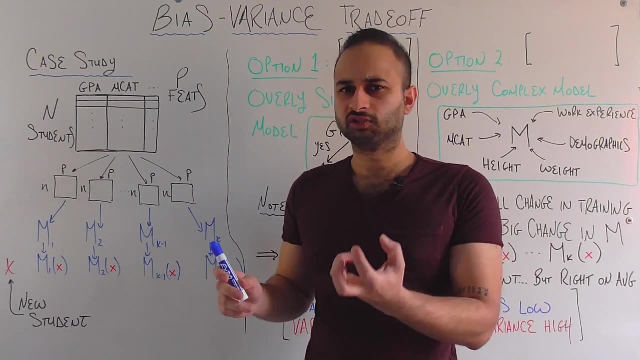 training data set K. you're gonna build a model called Mk. So, as we'll see in a moment, the crux of the bias-variance tradeoff is how similar these models are to each other and also how strong these models are in making a prediction about. 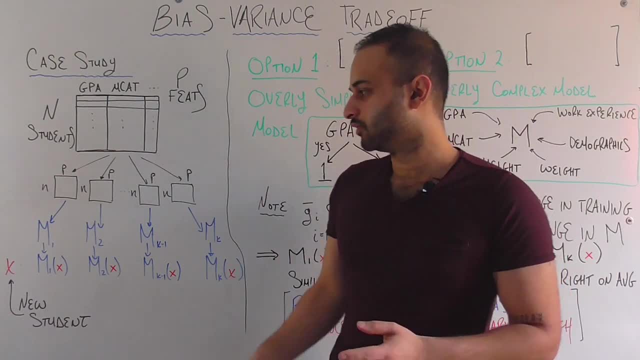 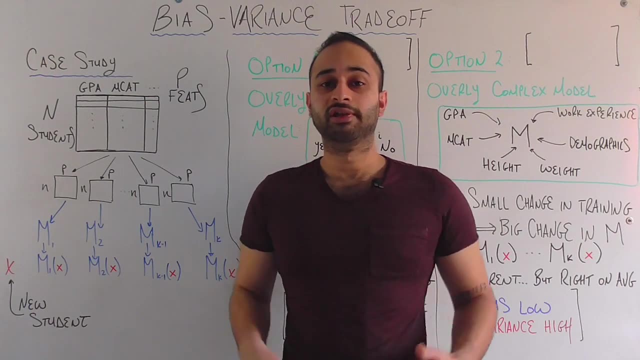 an unknown student. So, speaking of that unknown student, pretend you now get an unknown student X- this is some student not included in your data set- and you're trying to make a prediction about whether or not the student will be admitted to their first choice medical school. So let's say that you were given. 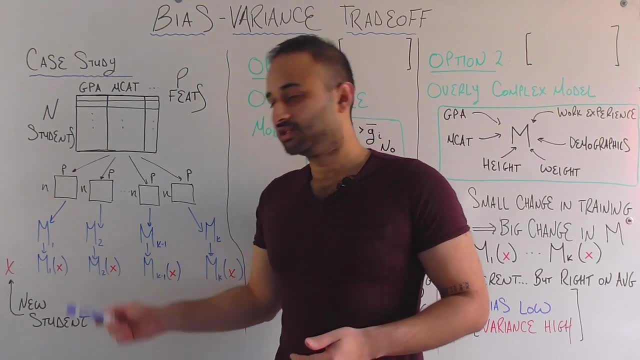 data set 1,, M2,. if you give you training data set 3, you're gonna get a model. you go ahead and say M1X. M1X is your prediction about whether or not this student will get into their top choice medical school. If you were, however, given training set 2,, you would use 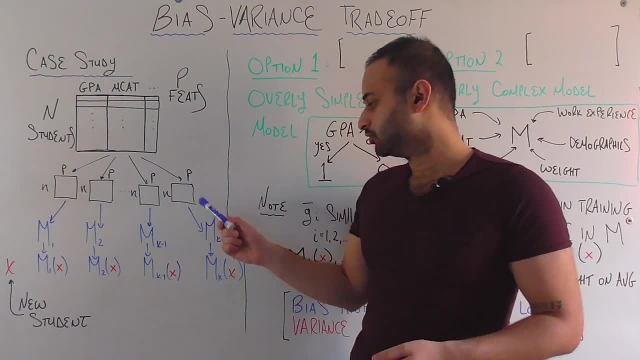 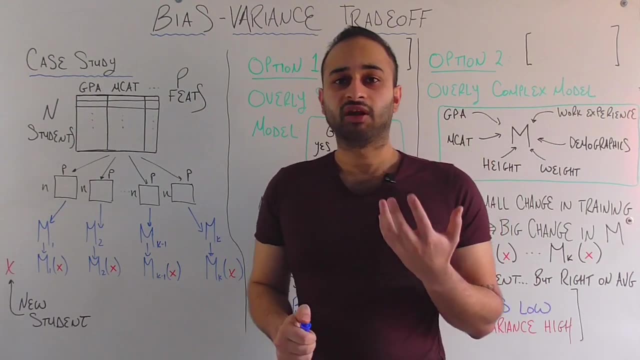 model 2 to make this prediction, and so on. If you were given training, set K, you would use model K to make this prediction. So hopefully this all makes sense. This is just some general machine learning framework, But let's now dive a little bit deeper and think about exactly how you build. 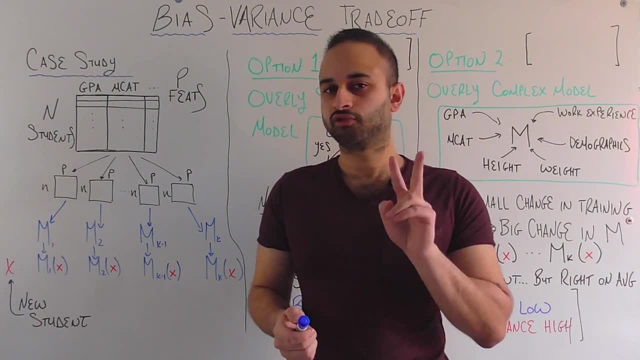 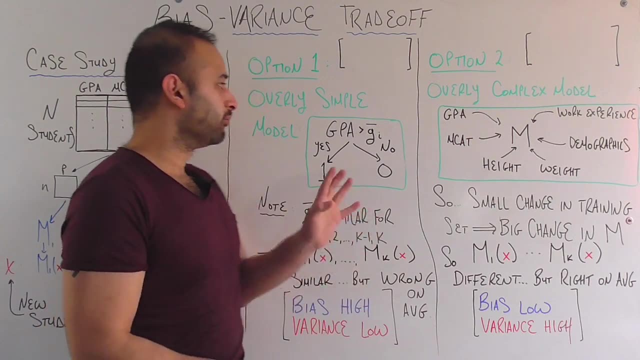 this model. So we're going to go over two big umbrella strategies and through these strategies we'll talk about the trade-offs that you have to make. So strategy number one is you build a overly simplified model. So, just to be concrete, that model, let's say, is only going to depend on 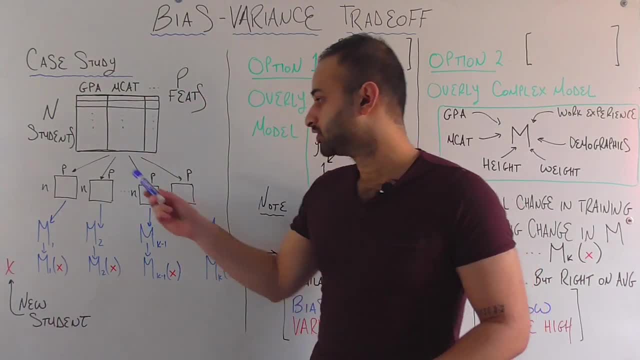 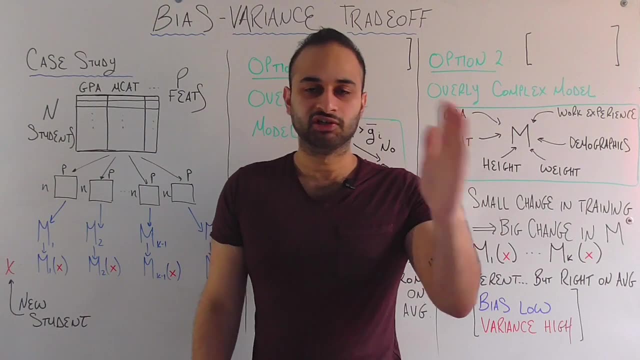 GPA. So just to be really clear, here's how you build those models. You take whatever training set is given to you. You compute the average GPA of all the students in that training set and your very, very dumb, very simple model basically says that: for an unknown student, 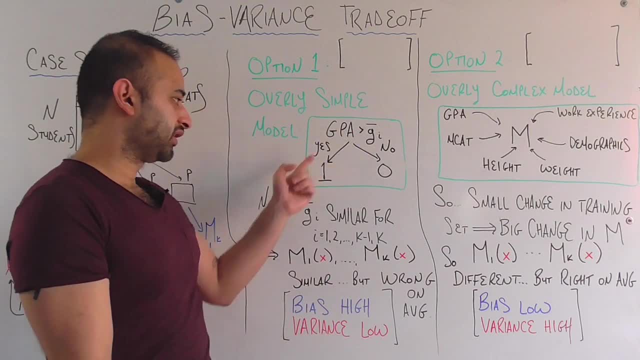 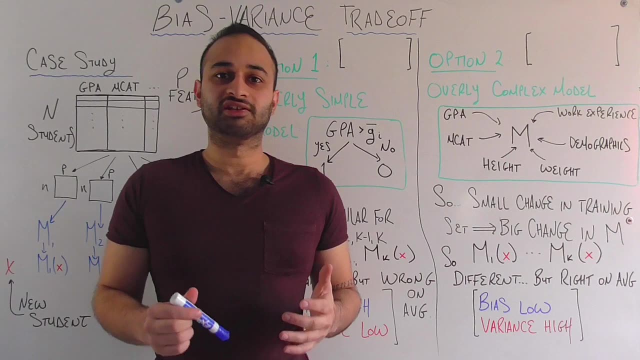 if their GPA is greater than that average, then you say that they are going to get admitted to their top choice medical school. So you take the average GPA of all the students in that training medical school. If their GPA is lower than the average, you say they are not. Now, obviously this 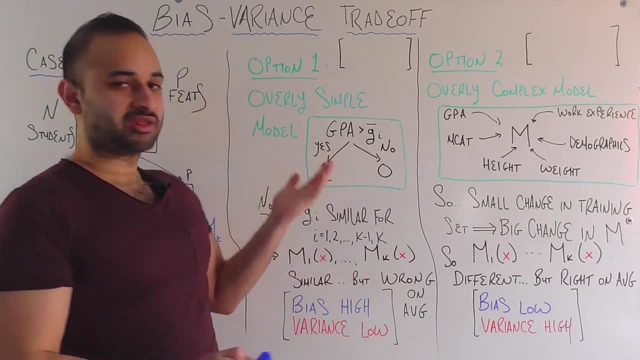 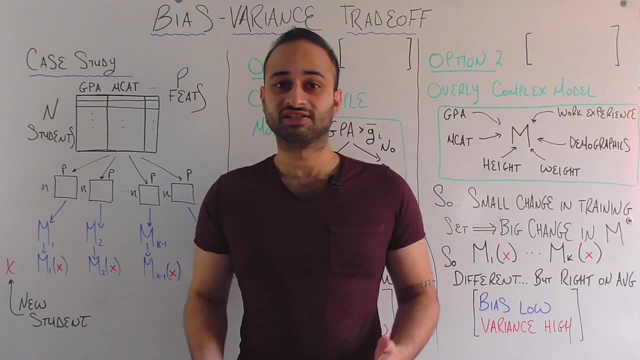 is not a great model for several reasons. The average GPA might not be the best predictor, but even bigger problem is you don't take any of the other predictors into account. Obviously your MCAT score matters, Obviously there's other things that matter, but your overly simple model is just 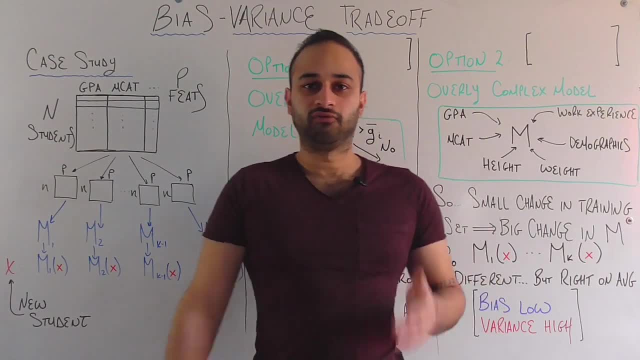 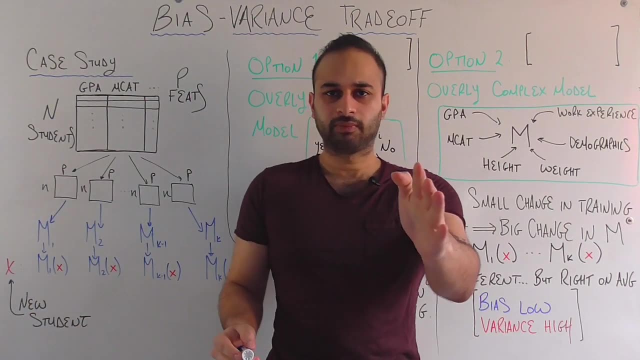 saying that whatever, just take the average GPA of the training set. If you're on one side of the cutoff, we're going to predict you get in. If you're on a different side of the cutoff, we're going to predict you don't get in. Now let's dive a little bit deeper and think about the exact 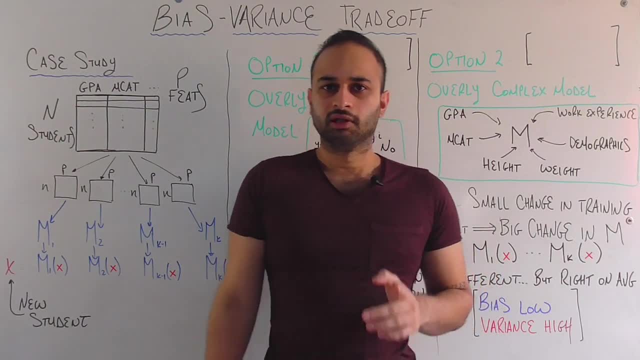 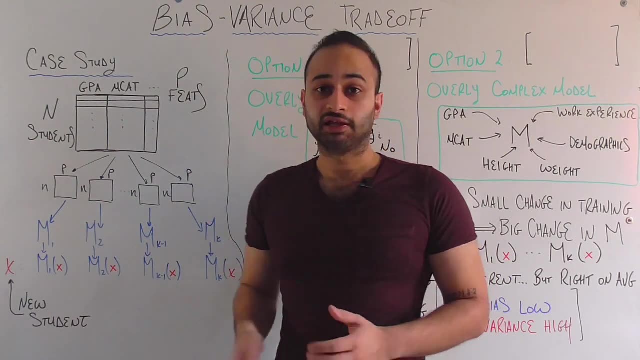 model you're building based on the training set that you get. Let's think about what the average GPA is going to be for each of these different training sets that you might receive from the medical board. Now, because each training set is completely randomized, truly random, the average. 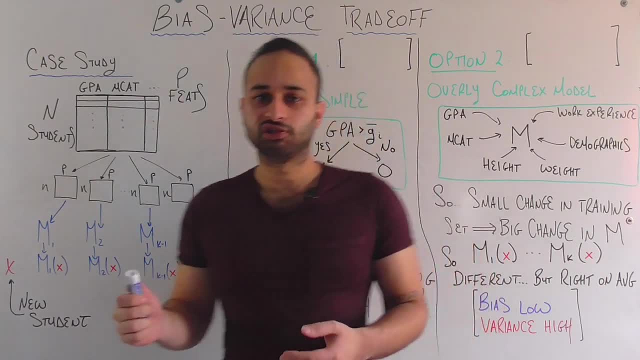 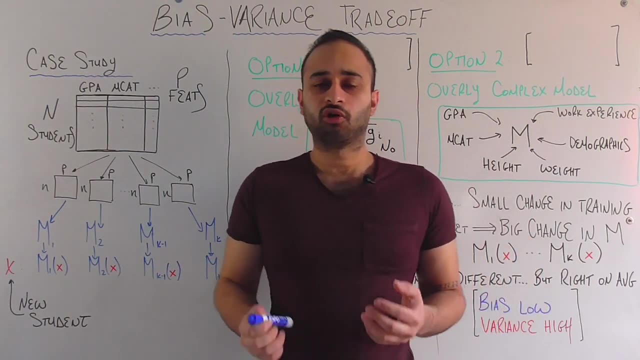 GPA is honestly going to be pretty similar in each of these, And since your very basic model here is only based on average GPA, that means that M1, M2, all the way to MK, are going to be models that are very, very similar to each other, right? Because they're only based on average GPA and 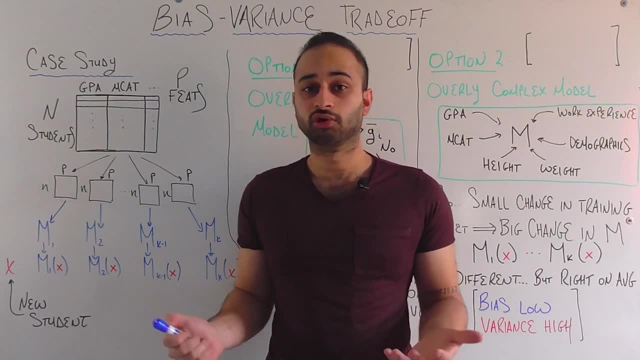 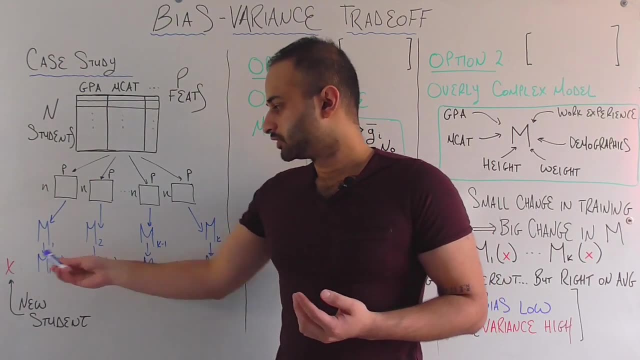 each of these categories is pretty much the same because they're truly randomized subsets of this overall set. Okay, so what that means for your models is that when you ask about an unknown student, they're all going to predict pretty much the same way, right, Because they're almost the 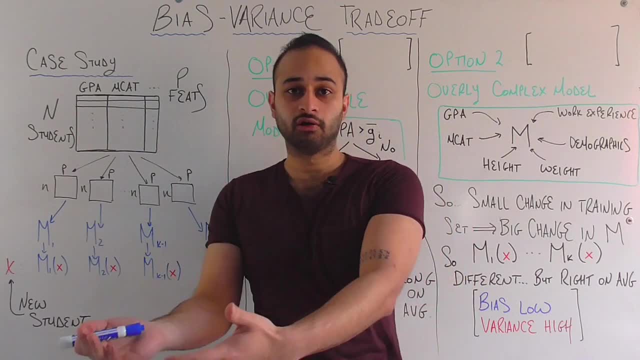 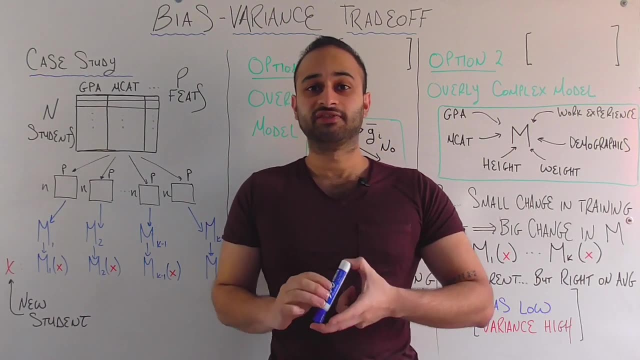 same model. So when you ask about the status of an unknown student, they're all going to give pretty much the same decision, no matter which training set you were initially given. What we call this officially in stats is that these models have low variance. What that means is that one model's 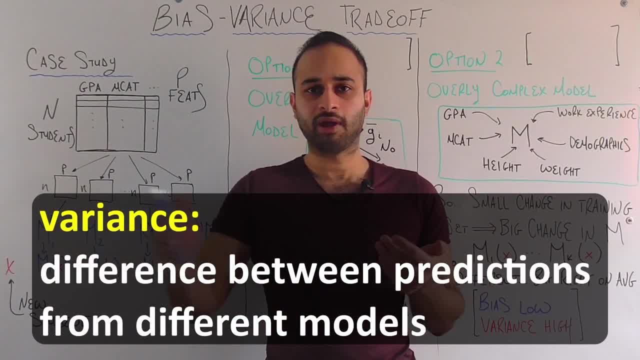 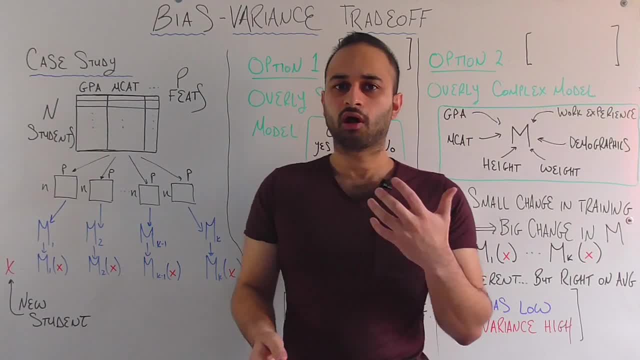 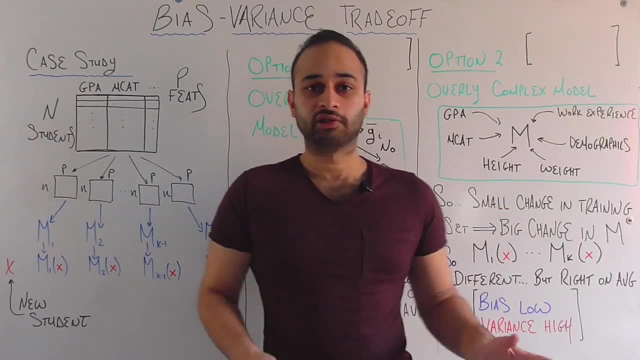 decision on average doesn't vary a lot From any of the other models decisions. they're all pretty consistent with each other, And this is actually something that we want in statistics. We don't want the model to change a lot based on little changes in your training set. So this is actually the good thing about this model. Now, 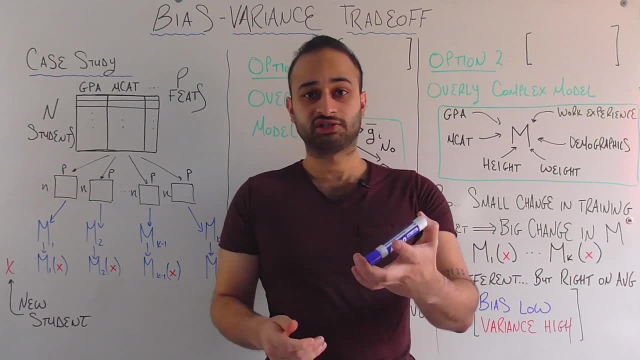 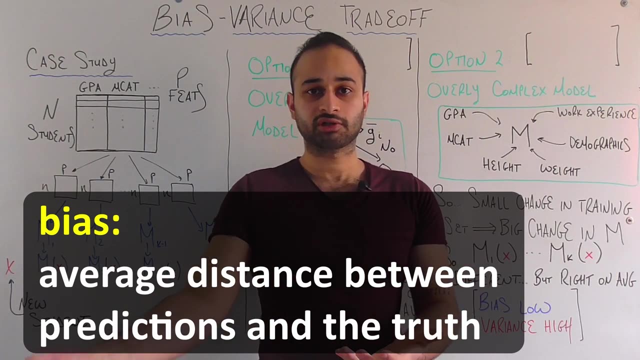 let's go back to the bad things about this model. This model, in official statistical terms, has high bias. Bias is the average distance of your model's predictions from the truth about this student. Now, since we know that this model is very basic, is probably not capturing most of the 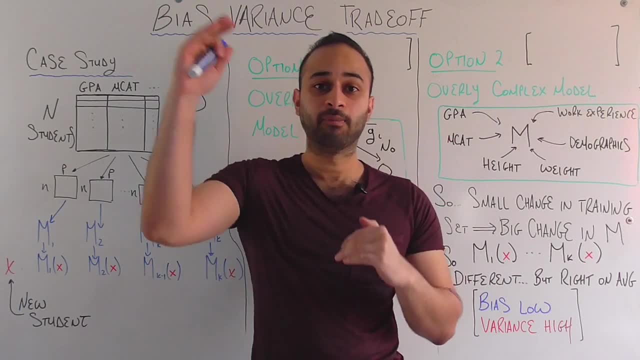 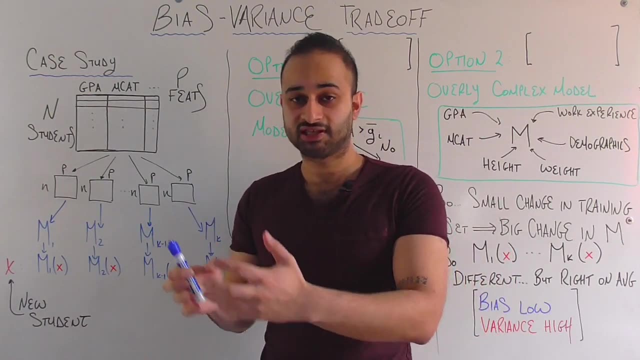 statistics in the admissions process, we would expect this model to have high bias. What that means again is that on average, even though all of these models are predicting pretty much the same thing, which is nice- they have low variance. they have high bias, which means on average they're not. 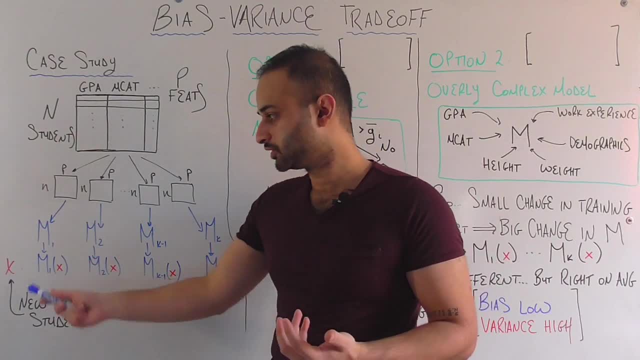 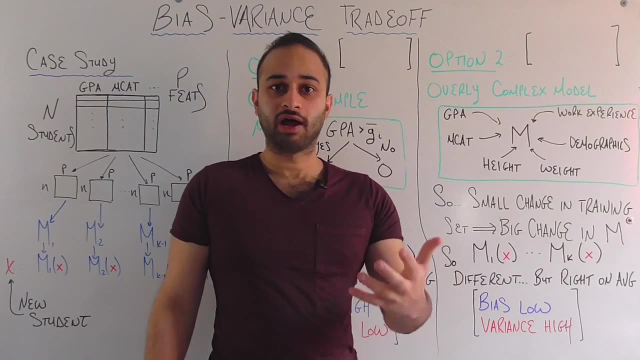 actually getting close to the true status of this student. So they're weak models in terms of bias, but they're strong in terms of variance. And another word that you'll see going along with this whole idea is underfitting. Now, if this sounds similar to a different word called overfitting, 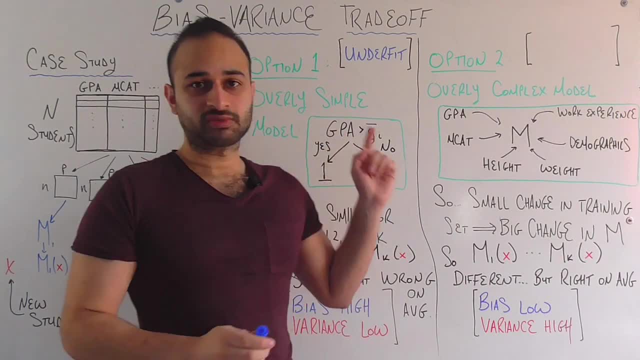 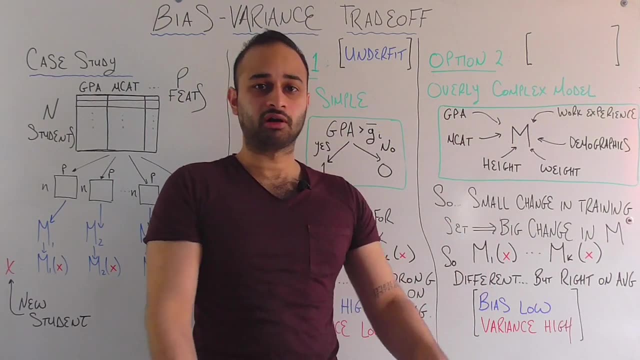 which we'll get to in just a moment. you have the right idea. This doesn't get talked about as much and I'll mention that in a moment. but underfitting is when you build a model that's way too simplistic. It doesn't capture all of the real patterns that are in the data. It's kind of dumb. 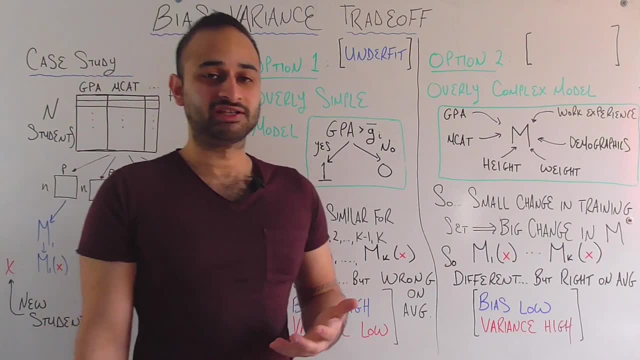 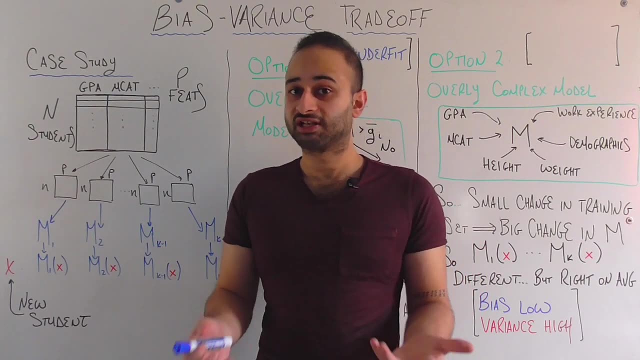 and that's what we're seeing here, But the one thing that it has going for it is that these models have low variance, which means that, based on the exact training set that you get, the model itself is not going to change a lot, which is nice, And so your predictions will at. 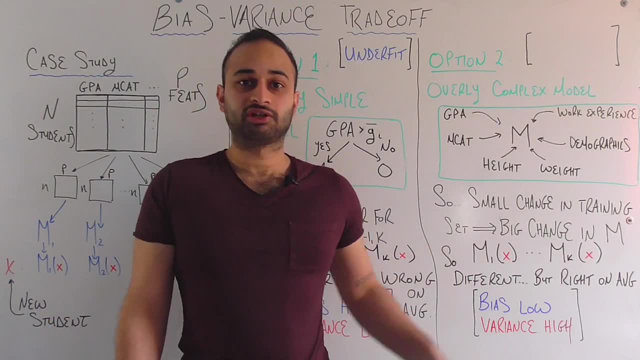 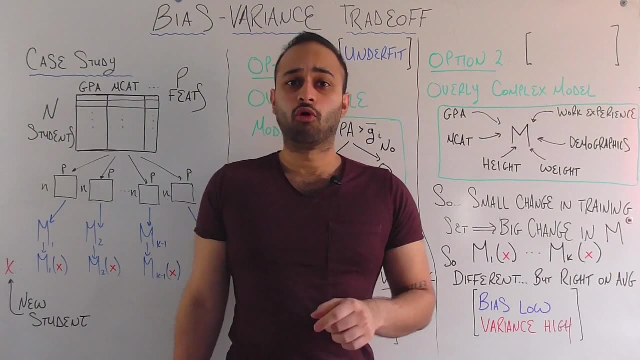 least be consistent, even if they're consistently wrong. Now let's go to the other case which I think people are more comfortable with, talk about a lot more, and I'll tell you the real world explanation for that in just a moment. But option two is to build an overly complex model. 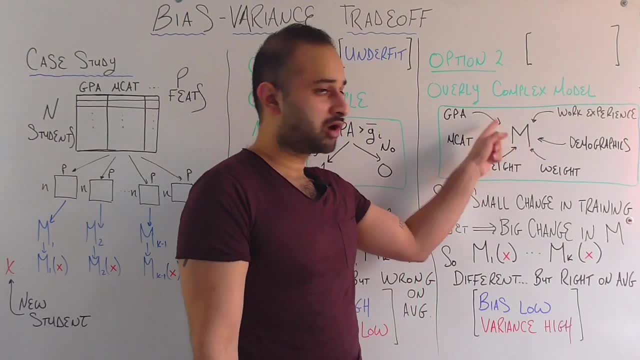 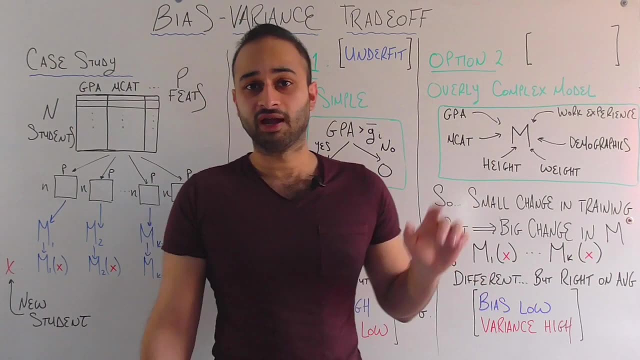 So I just kind of gave a picture of this here. We say that we're going to build some model M based on whatever training set that we get, and we're going to take into account everything. We're going to take into account the student's GPA, their MCAT score, their work experience, their demographics. 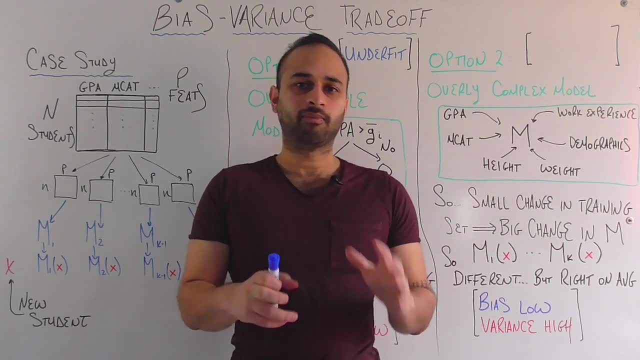 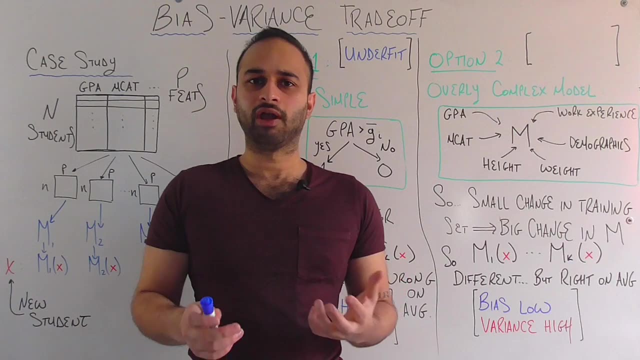 even stuff that probably doesn't matter, like their height and weight. And a complex model is not just one that has a lot of parameters, It's also one that incorporates these parameters in very, very complex, intricate ways. If you're building a decision tree, 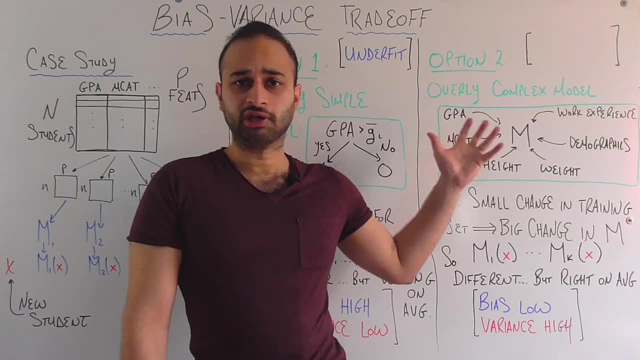 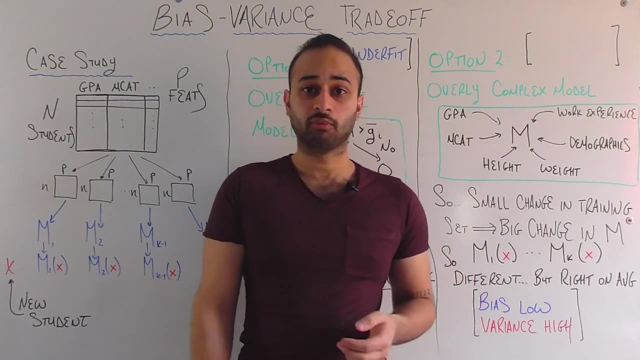 for example, and you're not careful and you let this tree grow too deep, then it's going to be overly complex. And what does it mean for a model to be overly complex? It means, based on the exact training set that you used in order to train the model. 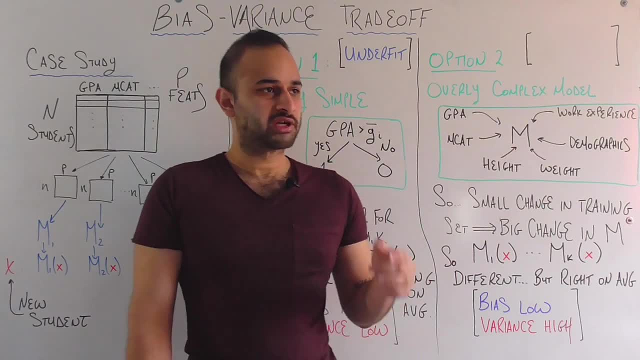 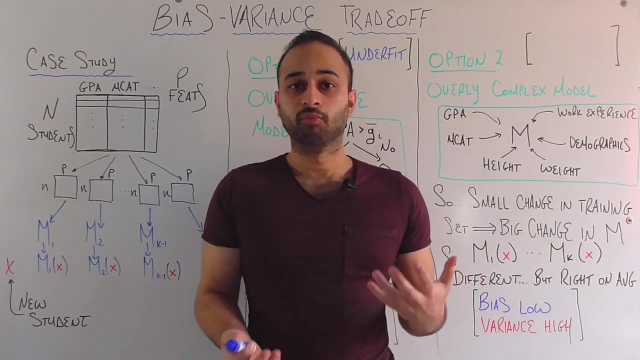 it's going to learn that training set too well. So of course there are very important, very crucial patterns in each of these training sets that helps us determine whether a student will or will not get in. But there's also a little bit of noise in each of these training sets. 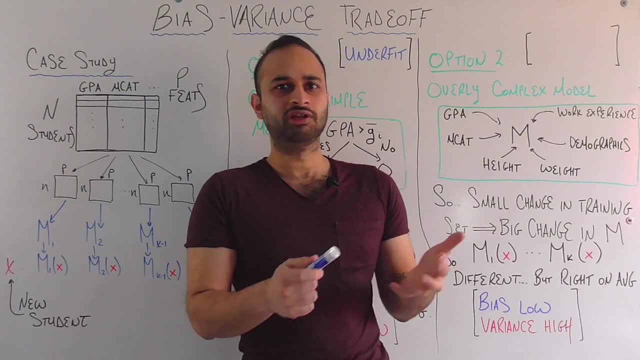 which means that there's some patterns that are going to be a little bit more complex, patterns that we could find, but they're not truly there. They're only there in the training set and don't generalize to the general population of students who are applying to medical school. 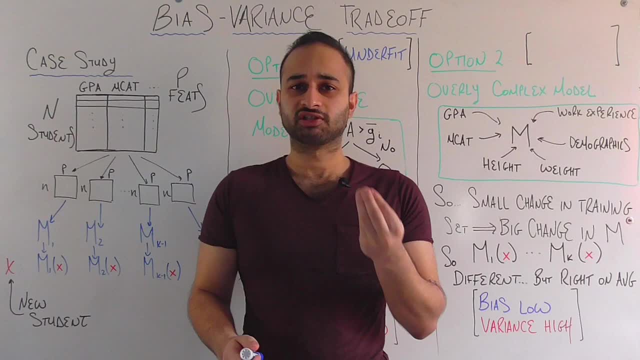 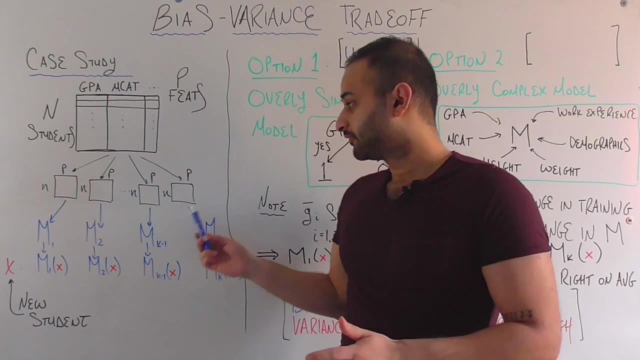 So an overly complex model is going to pick up on those patterns that don't actually exist. It's going to learn those and think those are important to it. What does that mean in real world terms? That means that, based on the exact training set that we're given by the medical board, 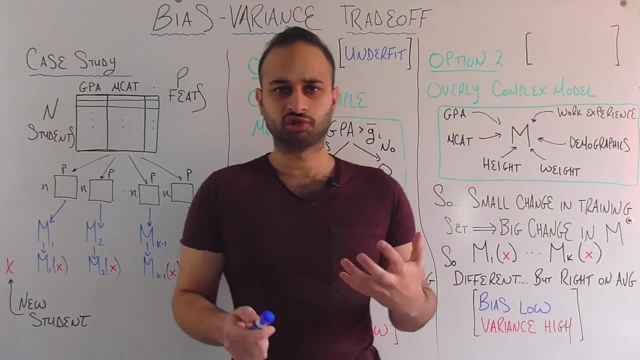 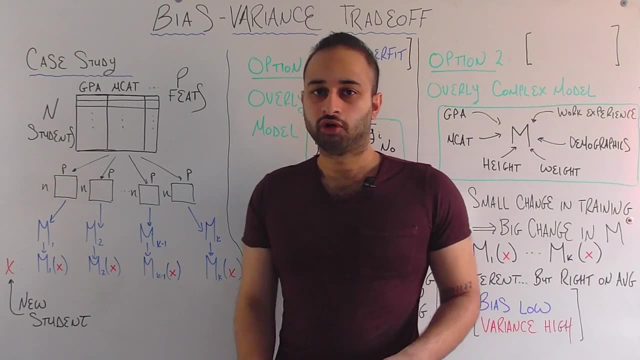 our model is going to change a lot, And let's think about why this is true just for a moment. Let's say that we get training set one. We're going to build some overly complex model. Now let's say that we get training set two. Training set two is going to have the same. 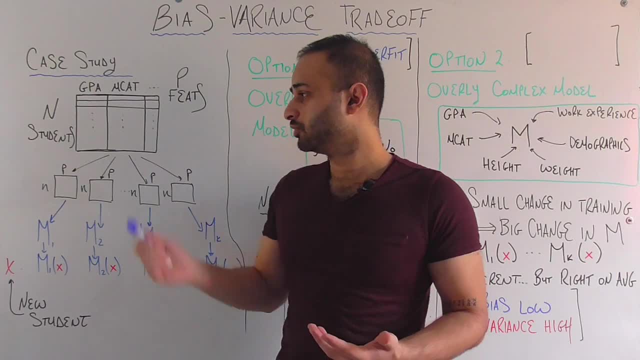 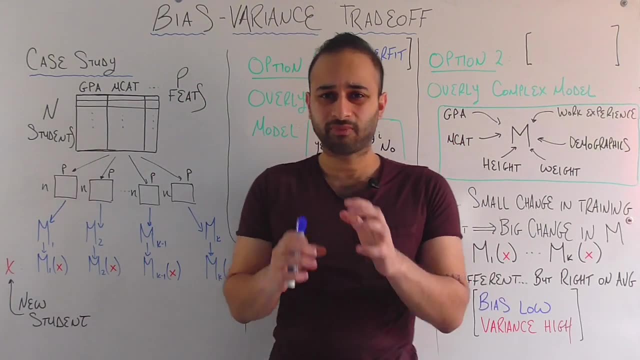 general idea as training set one because it's a random subset also. But because it's a random subset it's going to have a little bit of differences. But because our model that we build is overly complex, it's going to pick up on these little differences. think they're really 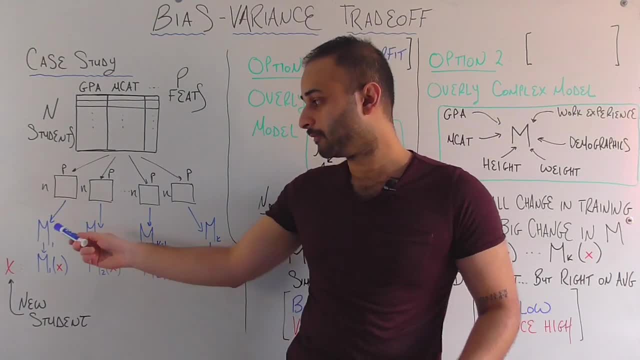 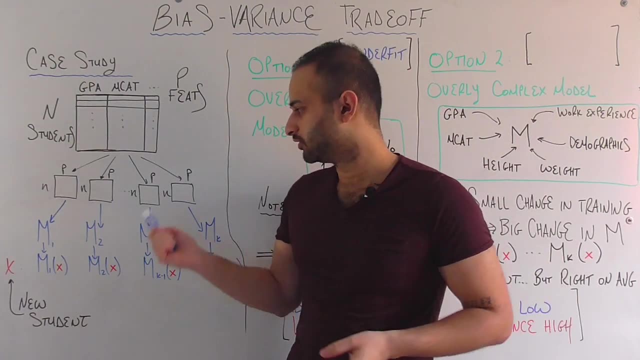 really important and build a model that looks nothing similar to model one. Similarly, for all of the training sets that we get, No matter which one we're getting- we're going to take that little bit of variation between the training set and the one before it and think it's a big deal. 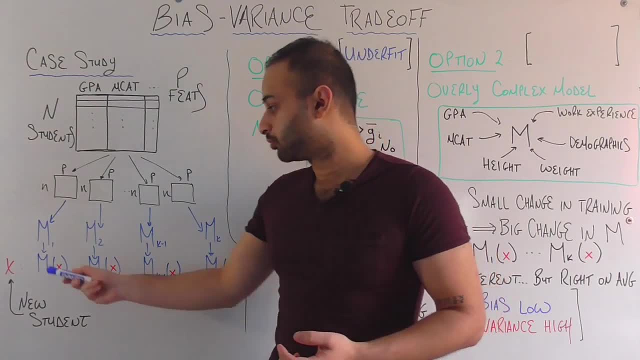 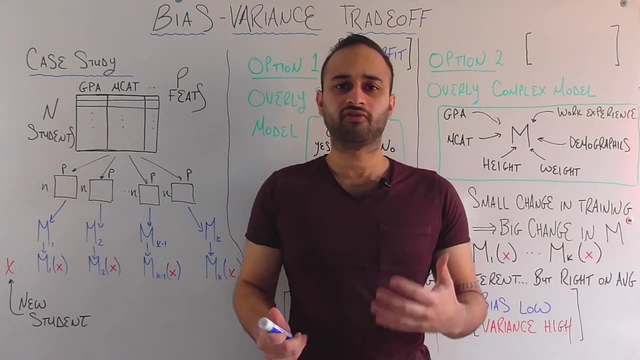 and build a very different model. What that means is now, when we try to predict this mystery student, we're going to get very variable results because these models are very different from each other, So they're going to give often very different outcomes. So model one might predict that the 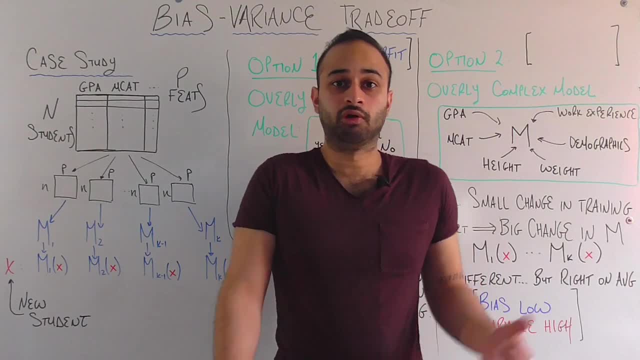 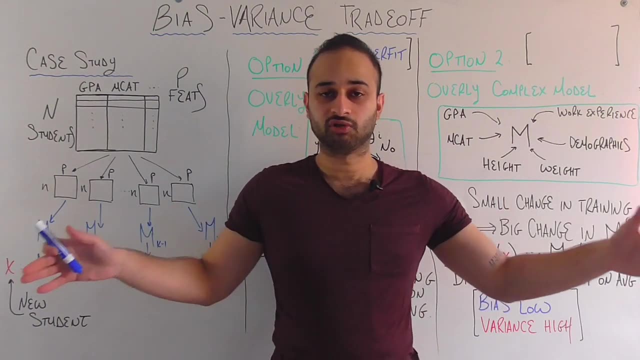 student will be admitted with high confidence. Model two might predict they will not be admitted with high confidence. Maybe model K predicts that they will be admitted with low confidence. There's not a lot of similarity between these models. Therefore we say: in this case we have high. 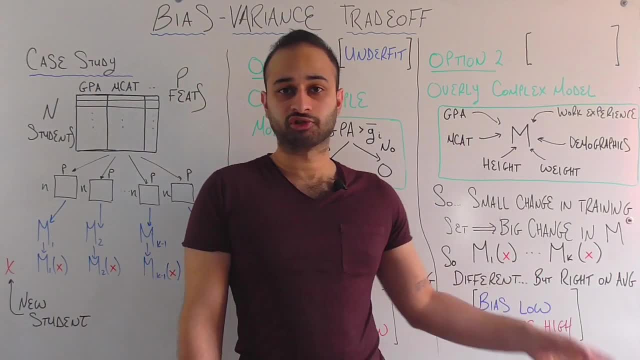 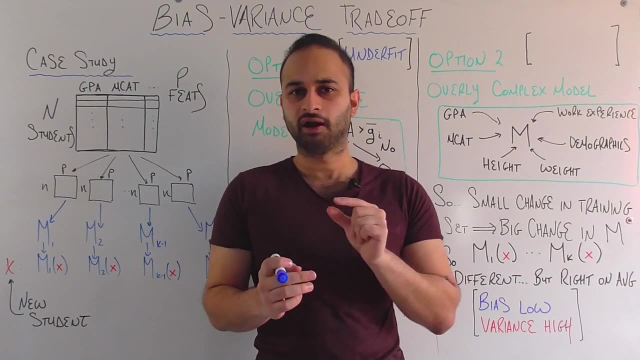 variance. But the pro of this strategy is that, on average, these models are correct. And let me try to explain this in real world terms. Although each model is learning little tiny patterns in the data that aren't really there, they are also learning the patterns that are there, And so, on average, these models are learning the 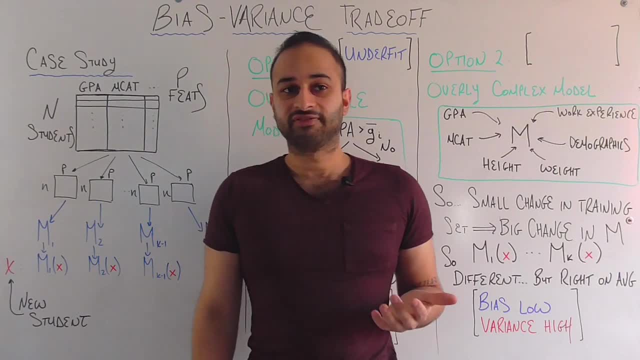 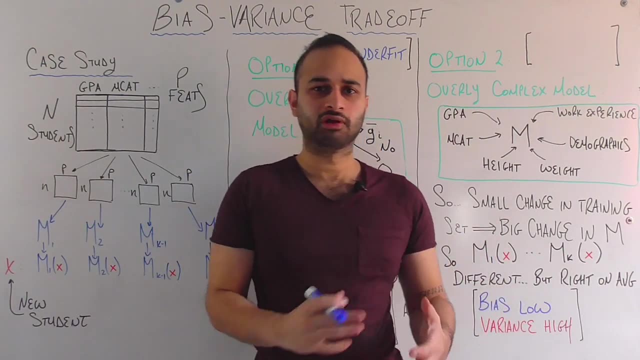 true patterns And on average they are correct. So just another way to say it is that they have learned the signal or the true pattern in the data. They've also learned the noise. So if we average over all of the models, we will get the right answer. But if we look at each model independently, 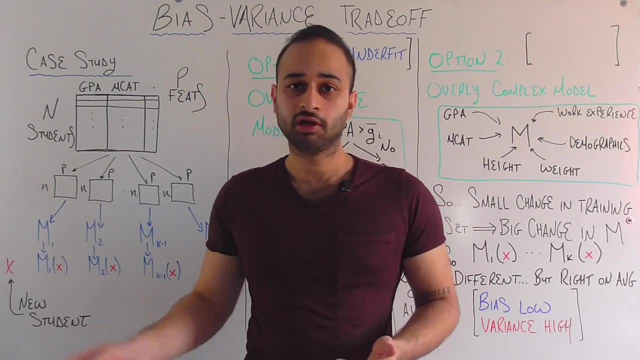 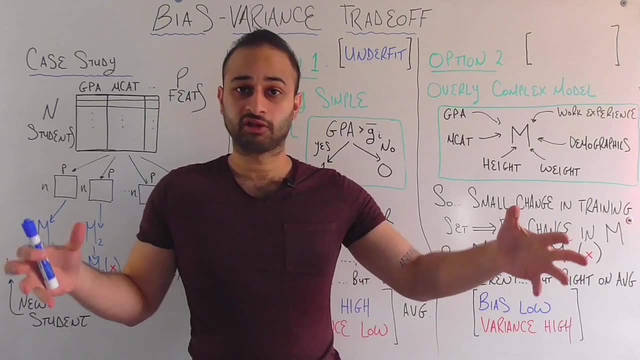 it's going to be pretty variable From the truth and pretty variable from each other. So what we say in statistical terms is the exact opposite of case number one, which is that these models have high variance, are different from each other but have low bias. Bias, again, is the average distance between 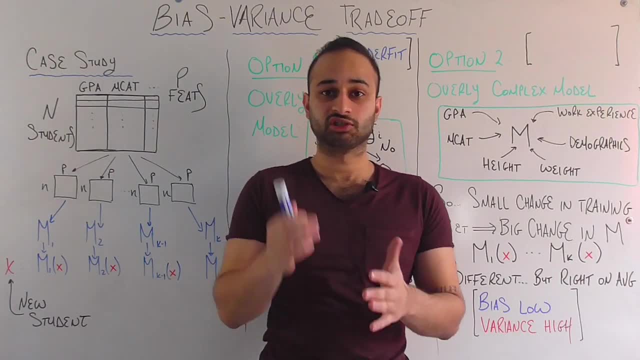 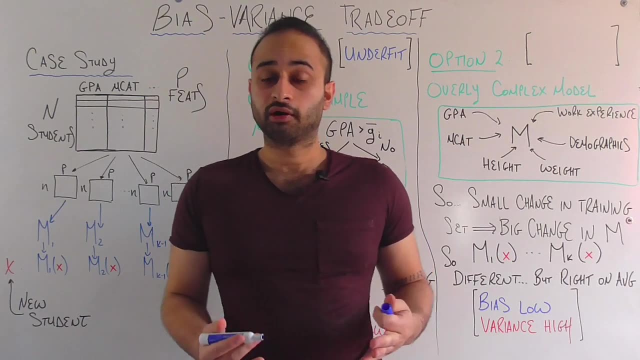 the prediction that the model makes and truth. So since that average distance is going to be small, averaged across all models, we say that we have low bias in this situation And the word that you've probably heard more is overfitting. So we say that these models are overfitted to the data. 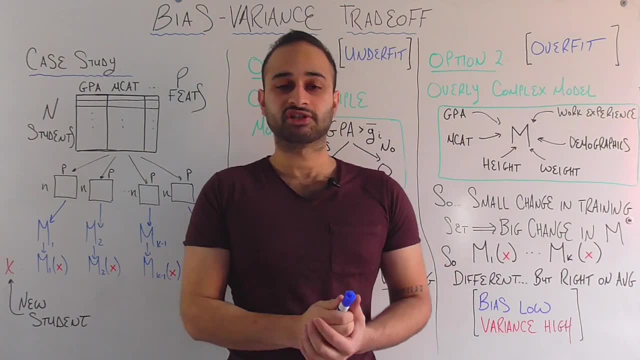 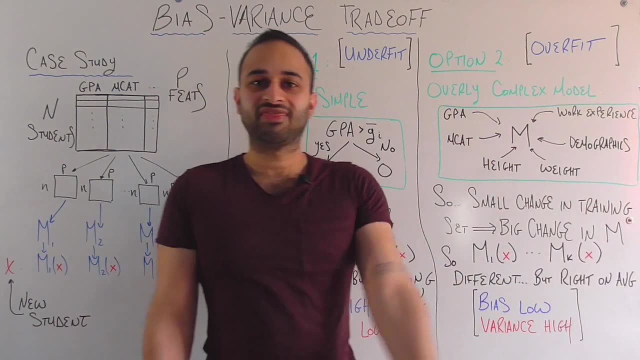 which means that they have learned this training data too well. So we have these two problems: underfitting and overfitting. So now, why do we hear a lot more about the overfitting problem? I think that comes down to the fact that nowadays we have programming. 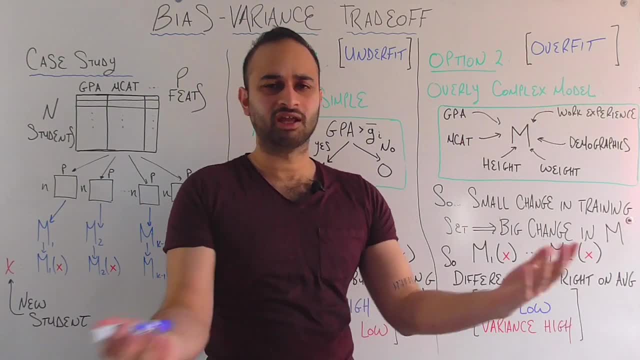 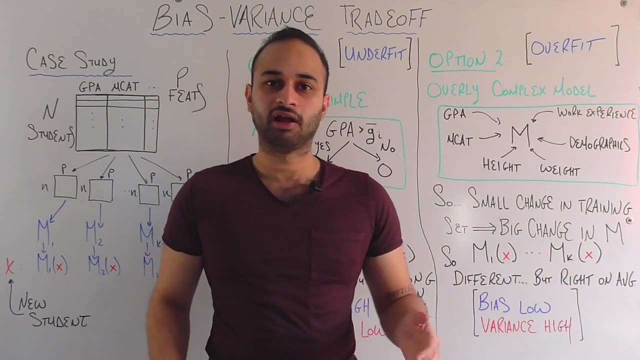 languages that are really accessible, which is great. We have like Python that anybody can pick up no matter which field you're in, which is amazing. But it also means that a lot of times people will just plug and chug. They'll get something from the internet. write three lines of: